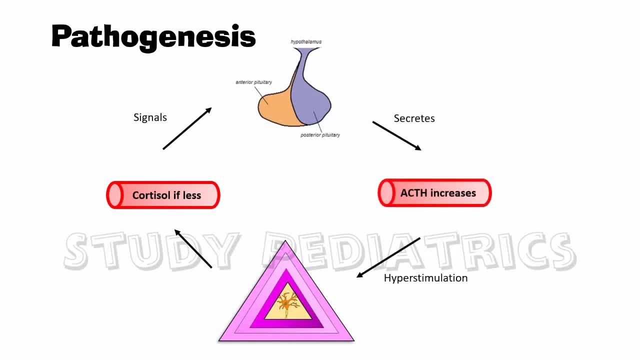 which stimulates adrenal cortex to secrete more cortisol. But due to congenital problem involving crucial enzyme deficiencies, the adrenal fails to produce cortisol. Hence, in response, pituitary secrete more and more ACTH, which causes adrenal gland growth, hence resulting in hyperplasia. 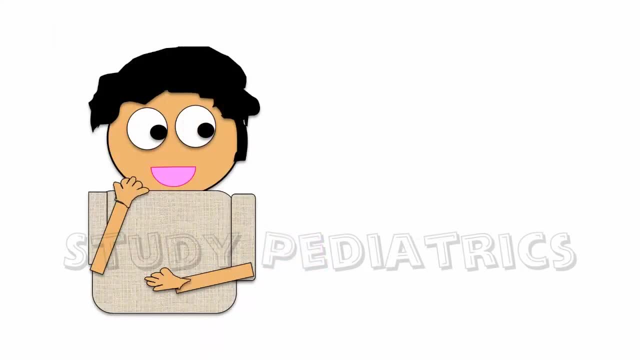 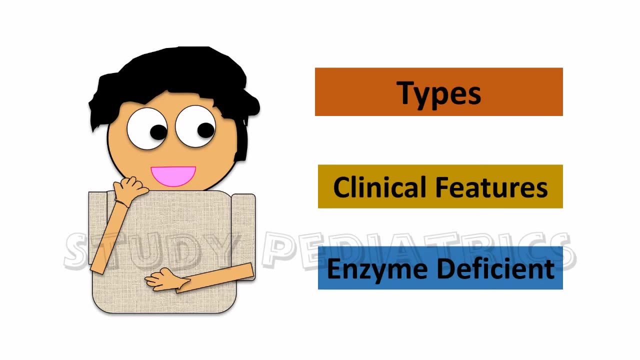 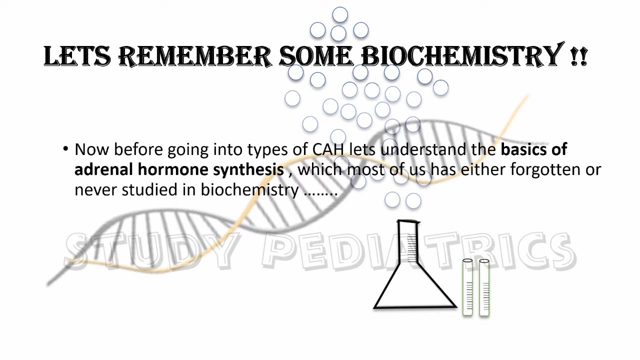 Till now we have seen as why we call the adrenals as hyperplasia, call it as CAH. Let's now look into types, clinical features and the enzyme deficient in it. But let's first remember some biochemistry. Let's understand the basic of adrenal hormone. 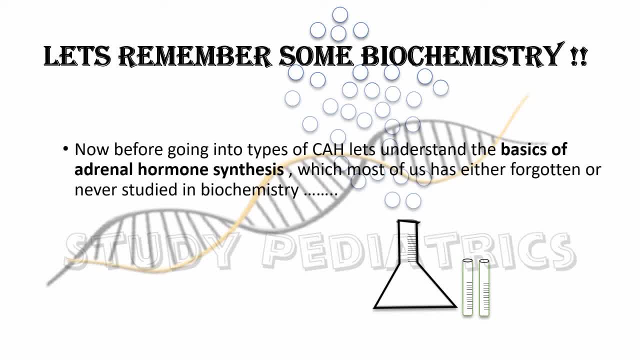 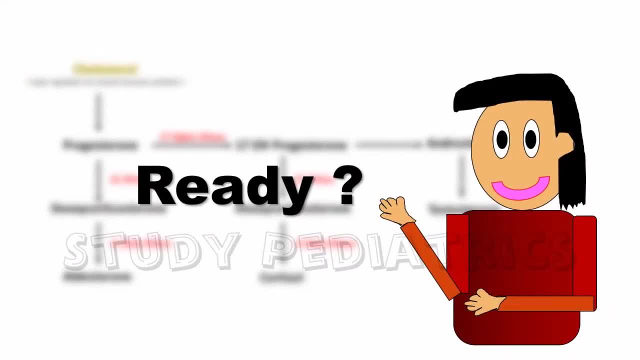 synthesis, which most of us has either forgotten or never studied in biochemistry. Here is the simplified flowchart of steroid hormone synthesis. This is indeed the simplest chart in cholesterol biochemistry. It is very important for us to understand it. Hence, please get. 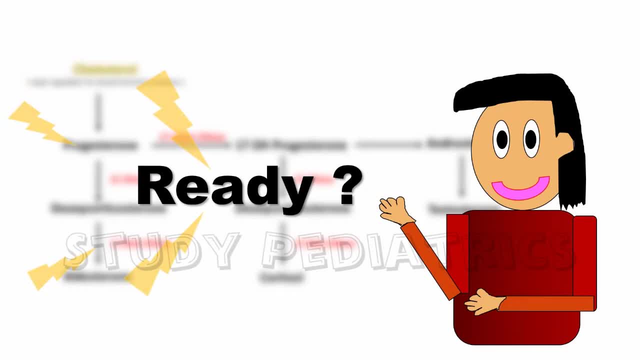 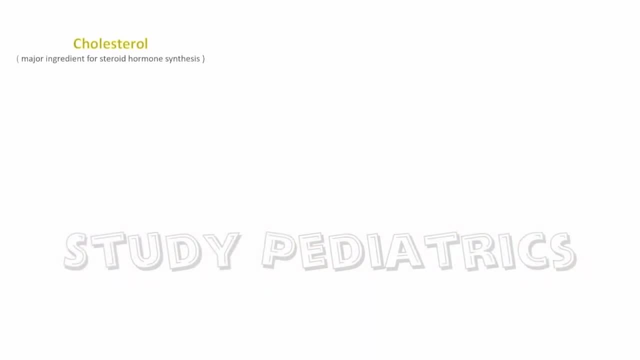 yourself supercharged before proceeding further. And I assure you, if you understand this chart, nothing will be difficult in this topic ever. Let's start. Cholesterol, major ingredient for steroid hormone synthesis. Cholesterol forms progesterone, which is the starting point of other compounds, Progesterone, with the help of enzyme 21-hydroxylase forms deoxycorticosterone, which later forms aldosterone. with the help of 11-beta-hydroxylase. With the help of 17-alpha-hydroxylase, progesterone forms 17-hydroxyprogesterone. 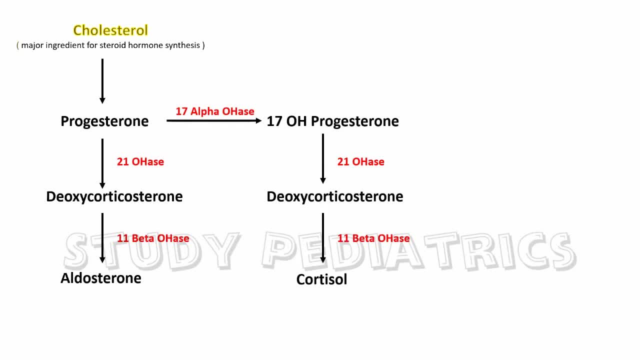 which follows similar path, like aldosterone, to form cortisol. as shown here, This 17-hydroxyprogesterone also helps in formation of androgens. Cholesterol- major ingredient for steroid hormone synthesis. Cholesterol- major ingredient for steroid hormone synthesis. Cholesterol, major ingredient for. 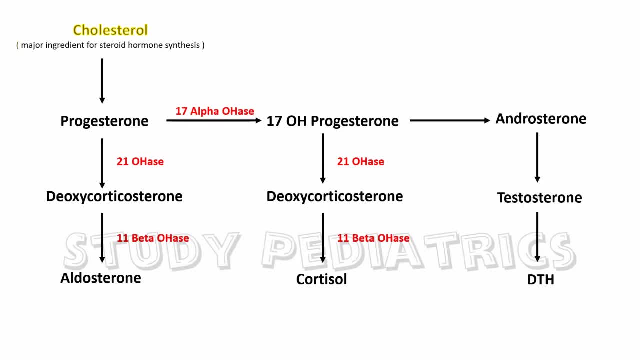 testosterone, a very common cause in this MATC. At the head it wines Motor MycosTER-ежде and would spasm baryosaccharin, lice-induced in the middle of the thyroid gland. The so-called noldosterone is most important vitamin that causes it's dependence, which is used by 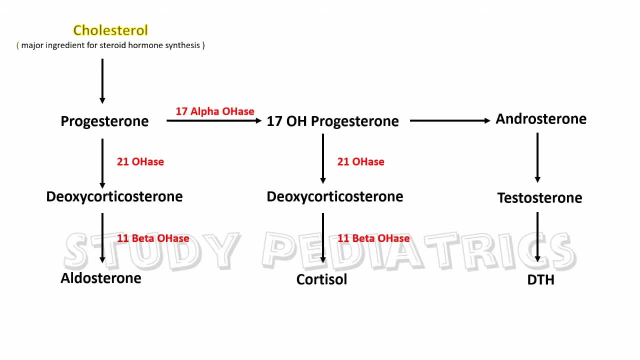 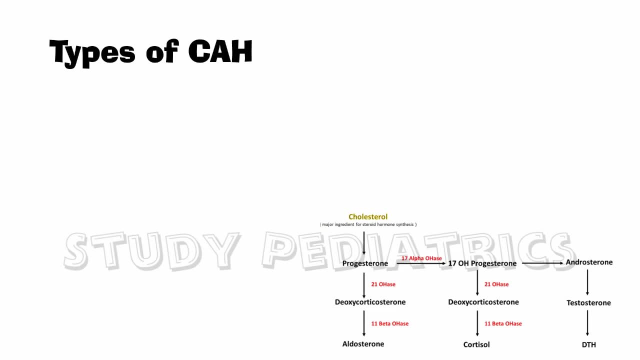 us toCAH injection, As we talked about the synthesis of steroid hormones, the type of are with respect to these enzyme- defines- deficiencies occurring in the pathway, hypoxylase deficiency, which is the most common cause of. 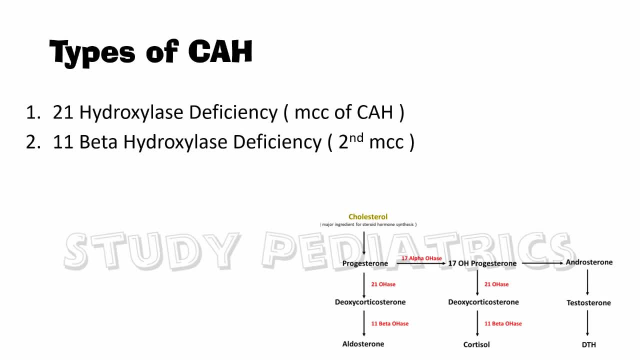 Second, 11 beta-hydroxylase deficiency, which is the second most common cause. Third, 17 alpha-hydroxylase deficiency. Fourth, 3 beta-hydroxysteroid dehydrogenase deficiency. And the fifth is aldosterone synthesis deficiency. 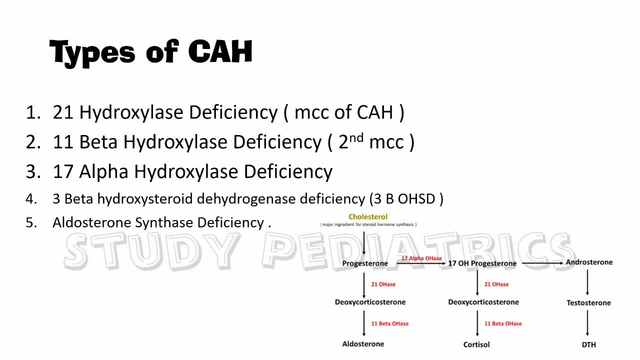 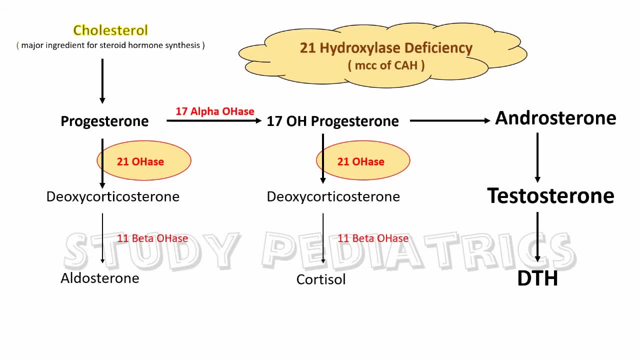 Now let's take first three, one by one. As we know, 21-hydroxylase plays an important role in synthesis of aldosterone and cortisol synthesis. hence there occur deficiency of both, Whereas since enzyme deficiency, the pathway gets directed towards androgen producing. 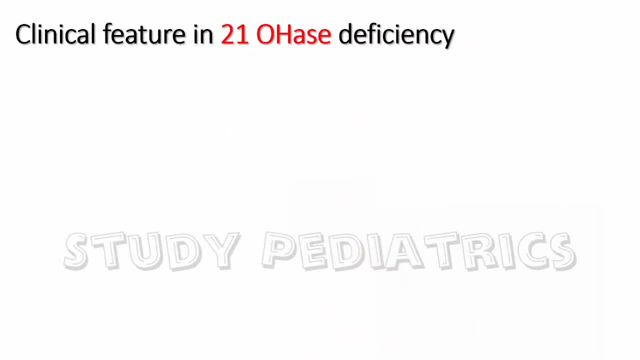 Now let's see the clinical outcomes of 21-hydroxylase deficiency. Since aldosterone is deficient, therefore less sodium retention and hence the BP falls, causing hypotension. And since cortisol level is less, hence there occurs drop in blood glucose level. 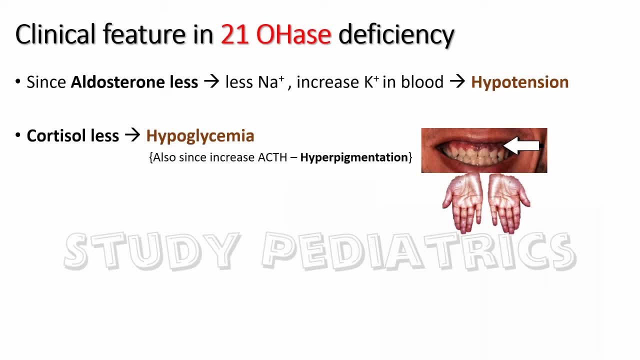 as cortisol levels drop And Stratozo היאzol is one of the major hyperglycemic agent, And In female, due to increased testosterone level. there occurs- they are occurs male like feature, such as virulism, ambiguous genitalia. 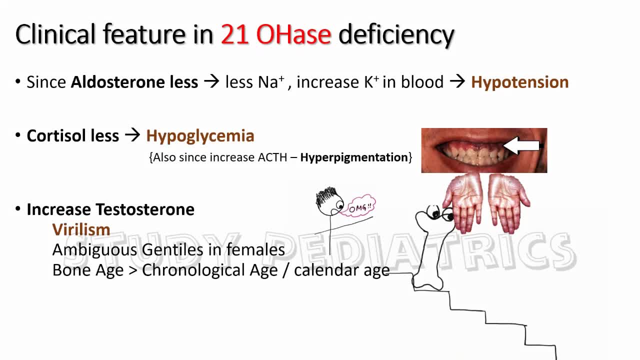 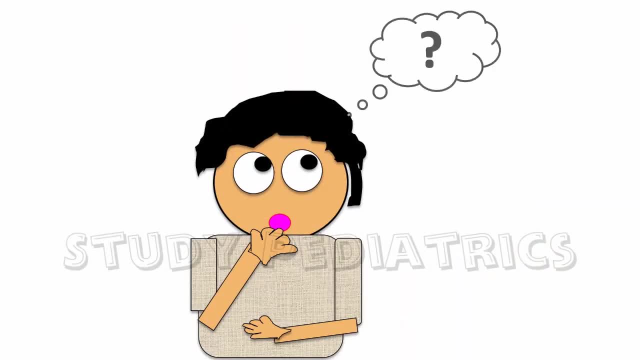 etc. Also since early closure of epiphyseal growth plate. hence bone age is more then chronological age. You might be thinking that if all the life-sustaining enzymes are especially same at the stage one of the majority in all the other people, 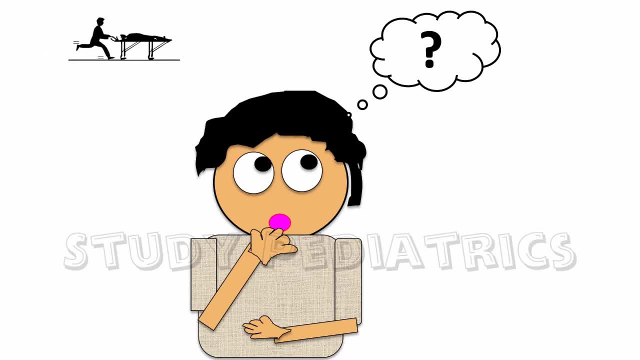 But end helped. So blood clot si not evaluated test result. These overalls are very popular, So none so risky. then how will the baby survive? Yes, you are right. Indeed, these babies land up in the emergency with the following typical history: as three weeks old child, 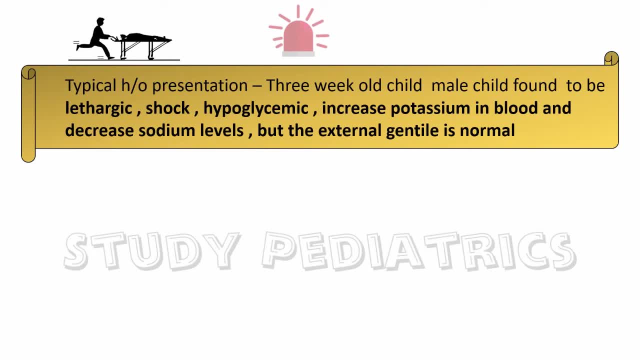 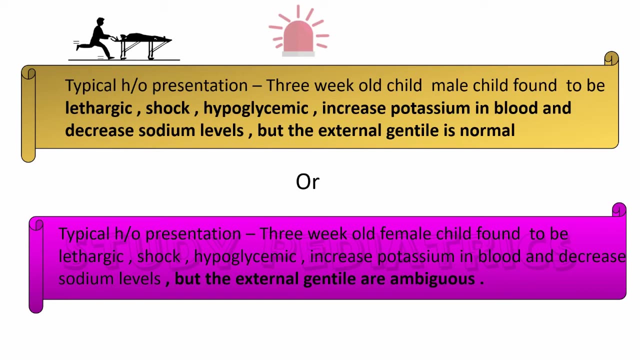 male is found to be lethargic, shock hypoglycemic, increase potassium in the blood and decrease sodium levels, but the external genital is normal or, in case of girl child, typical history of presentation is three weeks old. female child lethargic. 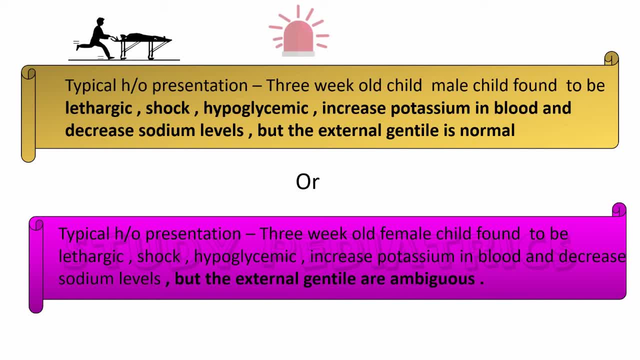 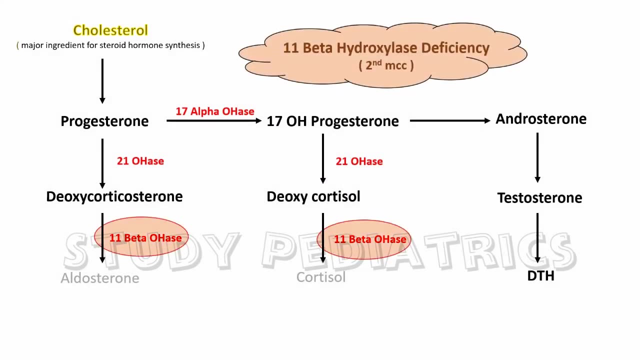 in shock, hypoglycemic, increase potassium in blood and decrease sodium levels, and the external genitals are ambiguous. Now let's consider the second cause of CAH, The second enzyme, that is, beta-hydroxylase deficiency. Here the situation is somewhat similar, but since 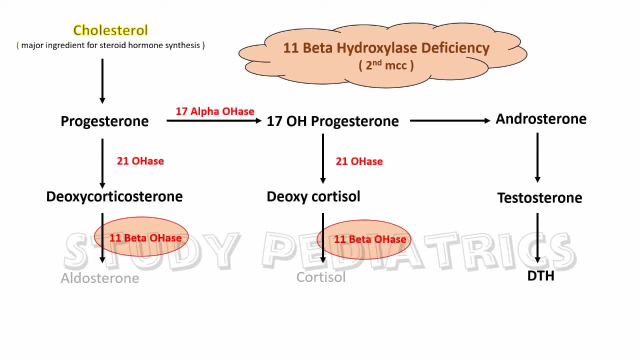 the terminal enzyme is deficient. hence there is formation of precursor like deoxycorticosterone and deoxycortisol, which can partially act like their final products. Hence the child here is more stable than previously taught. but as in previous, here too the androgens are increased. 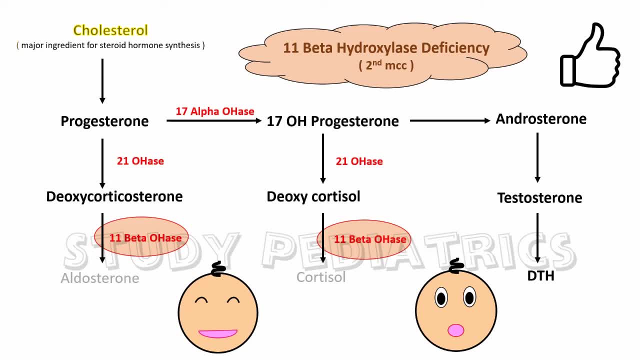 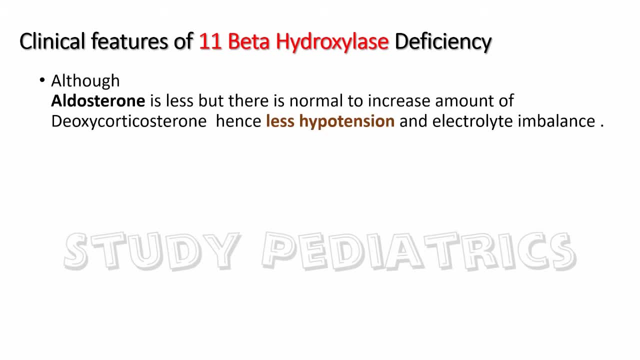 and hence ambiguous genitals are formed in a girl child. Now let's note these clinical features down, Although aldosterone is less, but there is normal to increase amount of deoxycortisol, Hence less hypotension and electrolyte imbalance. Similarly cortisol. 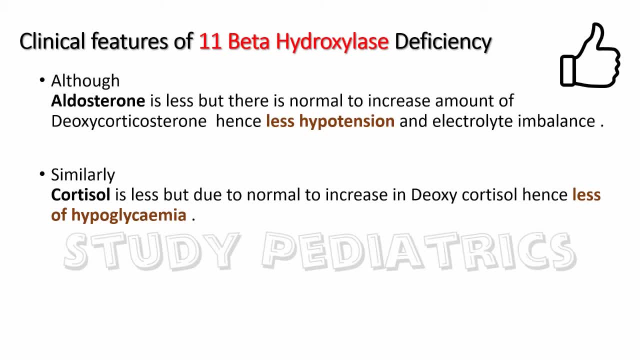 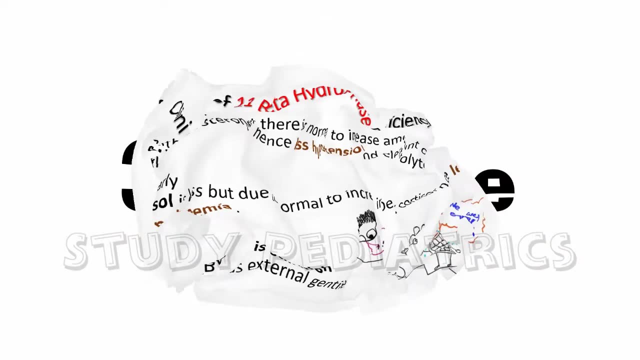 is less, but due to normal, to increase in deoxycortisol, hence less of hypoglycemia, but the testosterone is still high. Virilism, ambiguous external genitalia and bone age, more than chronological age, are seen. Now, coming to the third cause. or the third enzyme deficiency, leading to CAH 17 alpha hydroxylase deficiency, As we can see that 17 alpha hydroxylase has a role in cortisol as well as androgen productions. Hence there occurs shift of the path to aldosterone production. 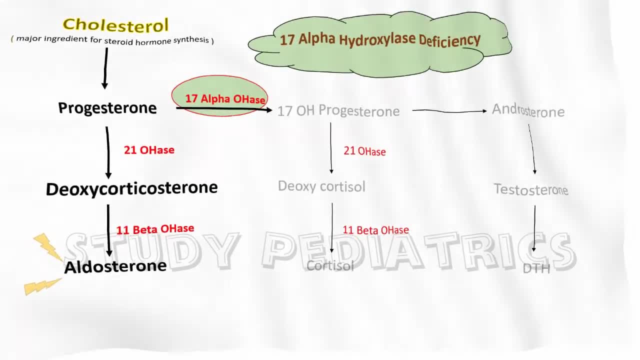 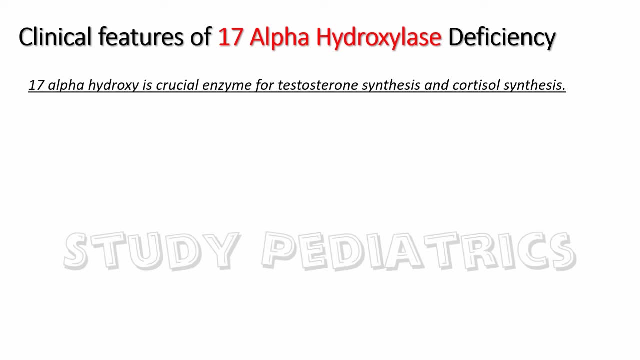 Let's understand further by considering the clinical features. As we know, 17 alpha hydroxy is crucial enzyme for testosterone synthesis and cortisol synthesis. Hence, decreased testosterone causes deoxycortisol. This causes ambiguous genitalia in males. Decreased cortisol causes less sugar in blood, leading to hypoglycemia. 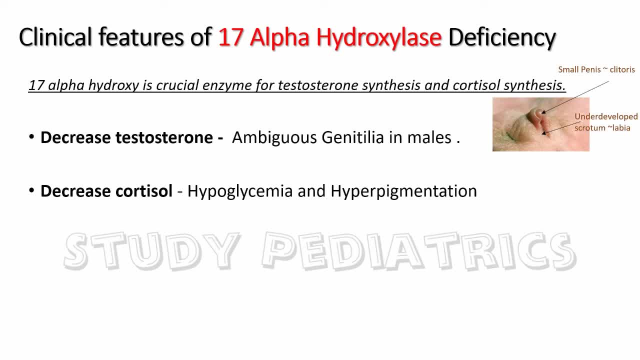 and also there occurs overproduction of MSH due to common pathway between ACTH and MSH synthesis, resulting in hyperpigmentation, And increased aldosterone causes sodium water retention, leading to hypertension. Now let's see how we can manage a patient with CAH. 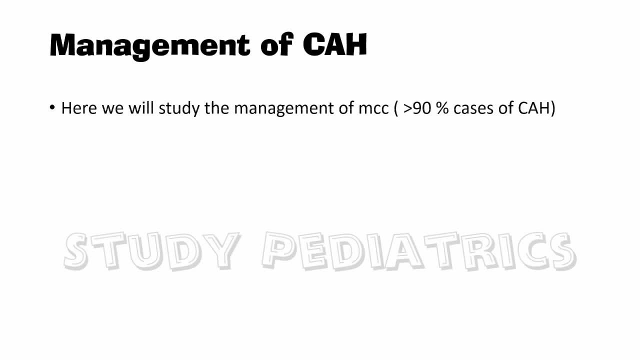 Management of CAH. Here we will study the management of the most common cause, that is, more than 90% of the cases of CAH, which is 21 hydroxylase deficiency. The drug of choice is hydrocortisone, which is given lifelong with addition of.